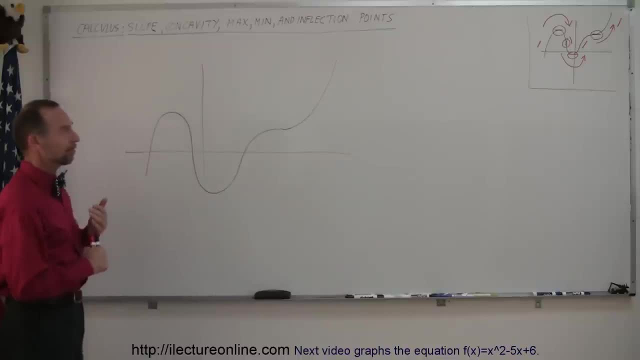 inflection points And before we get all started on that, let's make sure we understand what those things are. So what I've done is I've put on the corner there a little graphic we can reference later. But I want to go over that very same curve. this is the same curve, a little blown up here. 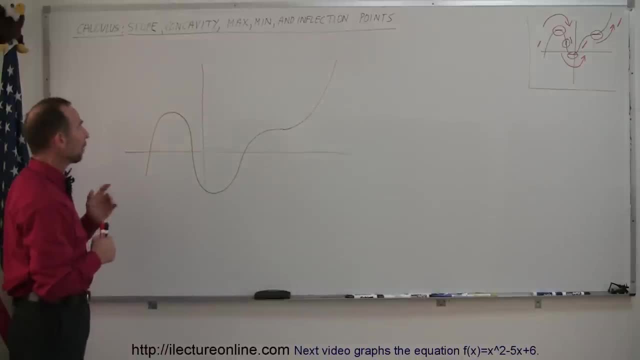 and I want to indicate to you what all these various things are. So first of all, slope. The slope is the steepness of a function at particular places. You can see that from here to there the slope is positive because it rises as you go to the right. So here we have a positive 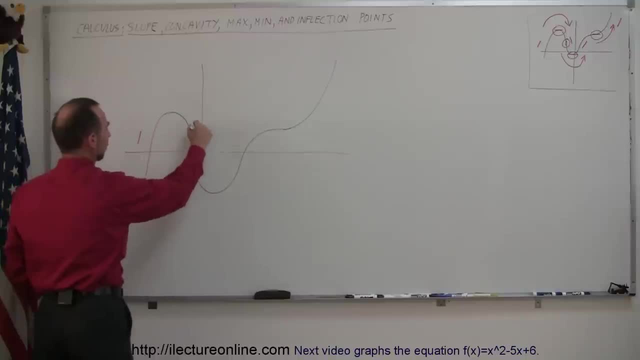 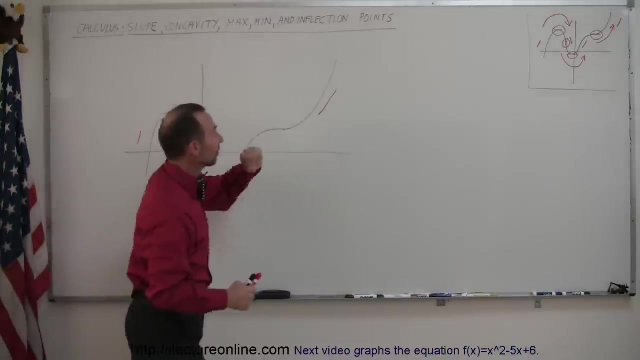 slope Over here. from there to there, we have a negative slope. From there to there, we have a positive slope. there to there, we still have a positive slope. So slope is simply the derivative of a function, and here you can see that the slope is positive. there's negative, positive and positive. All right. 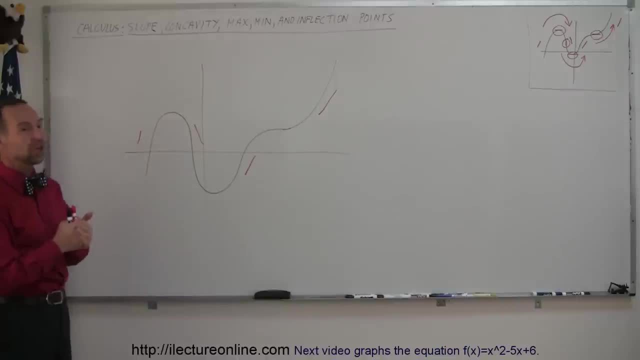 concavity. Concavity is how the slope changes. You can see that from there to there the slope goes from positive to negative. So the slope goes from a large slope to a small slope, to a negative slope. So they call this concave down. So this is considered what we call concave down. 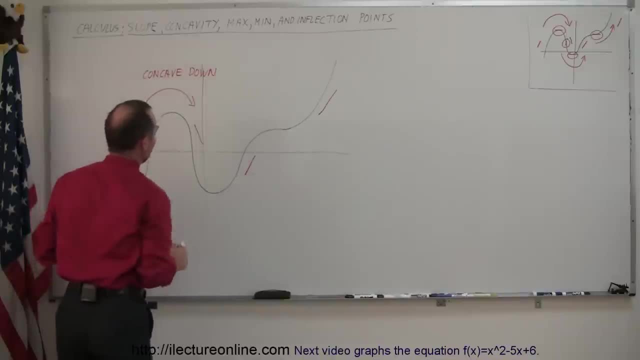 And then here in this region, right here, we go from negative slope back to a positive slope, So the slope increases there. So they consider this region here on the curve to be concave up, And then over here the slope is changing from there to there. So we could say that this is 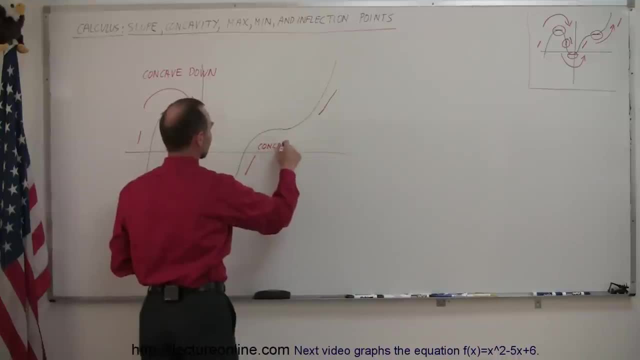 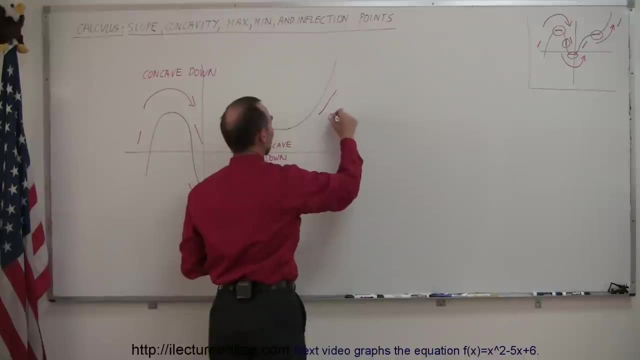 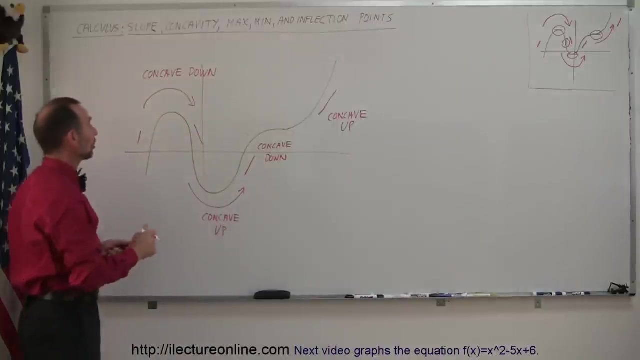 concave down. And then over here we consider that this back is concave up. So the concavity of a curve simply explains how the slope is changing. Is it becoming smaller Concave down? Has it become bigger Concave up? Smaller Concave down, Bigger Concave up. Then we also have points on the slope. 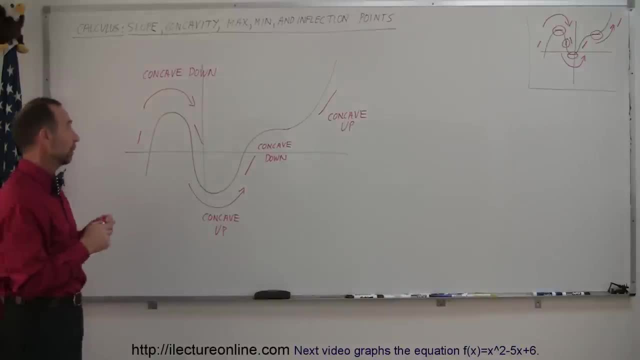 I'm sorry, points on the graph where the slope is zero. So when we top out here at the very top, you can see that the slope is zero And if it's, if the slope is positive here and negative there, that's a maximum point on this. 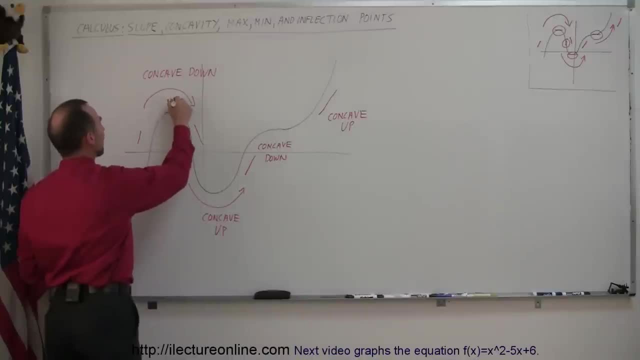 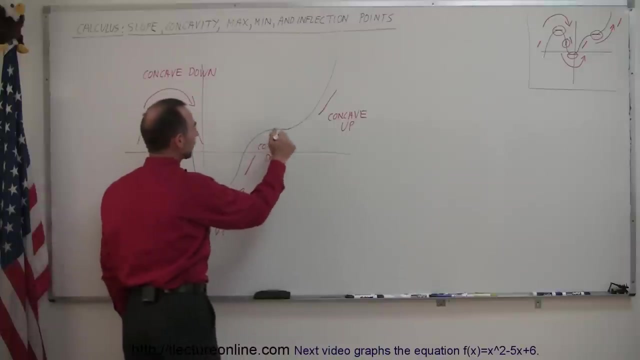 curve in this particular locality, So this is considered a maximum, or a local maximum point on the graph. Over here you can see that it bottoms out. The slope over here is zero And so this is considered a minimum point on the graph. And then, if you look over here, you can see that the slope 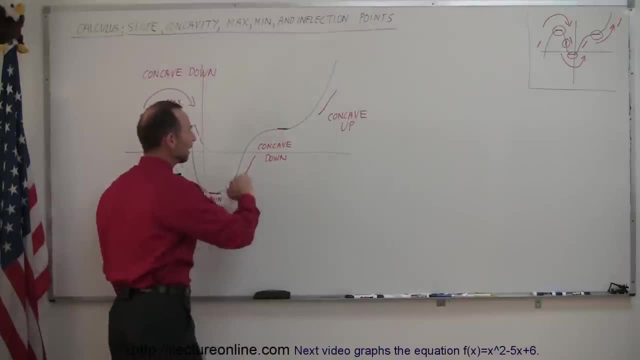 here is zero again, But in this case it doesn't. it's not a maximum or minimum. even though it gets bigger, then it levels off and then it continues to get bigger. This is not considered either a maximum or a minimum. This is what we call a an. 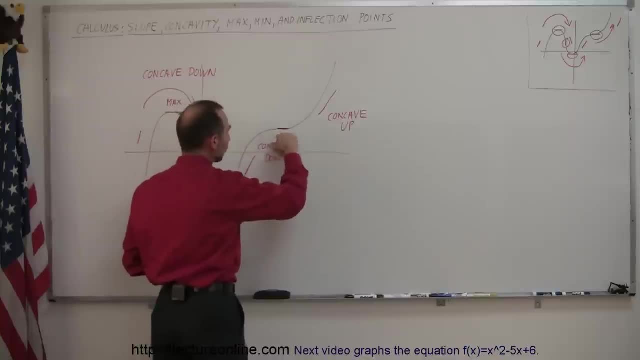 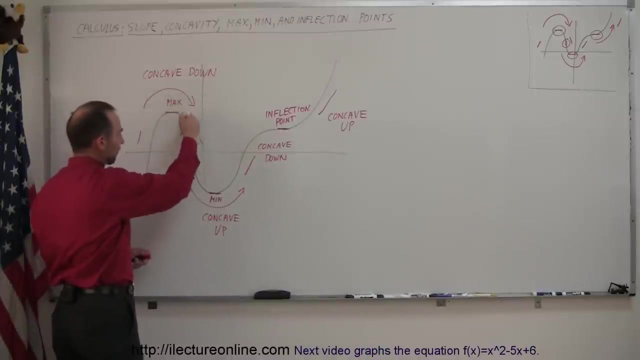 inflection point, So where the slope is decreasing and then slope becomes increasing again, we call this an inflection point. and if you look at another place here again, here we have a region where it's concave down, and here there is a region where it's concave up, where this changes right in the middle. here that is. 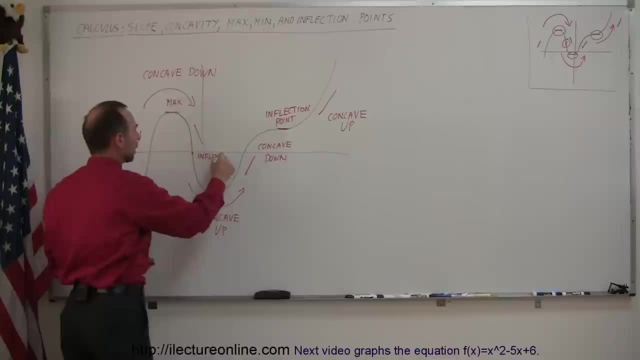 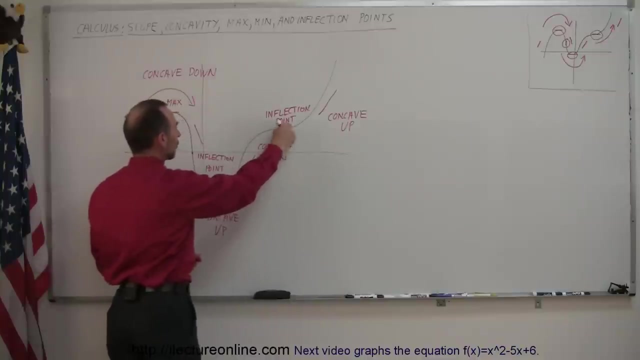 also called an inflection point. there's one fundamental difference between these two inflection points. this inflection point: right here there's no max or min value, meaning the slope doesn't go to zero. over here the slope does go to zero. so make sure there's a very big 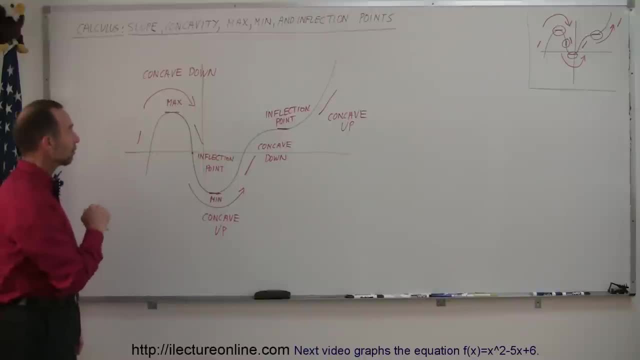 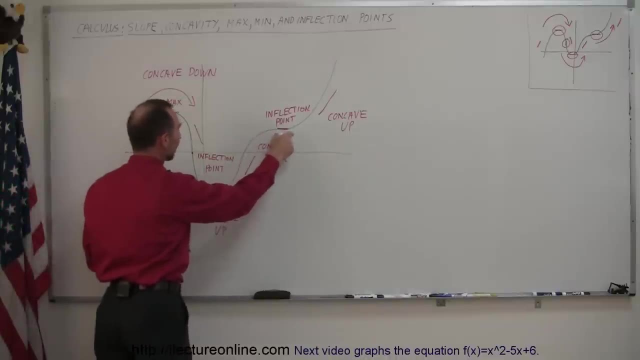 difference. you see the difference between those two inflection points. if we're trying to find the point on the graph where the slope is zero, we'll find the point over here, we'll find a point over there and we'll find the point over there. this point will not be found by finding the places. 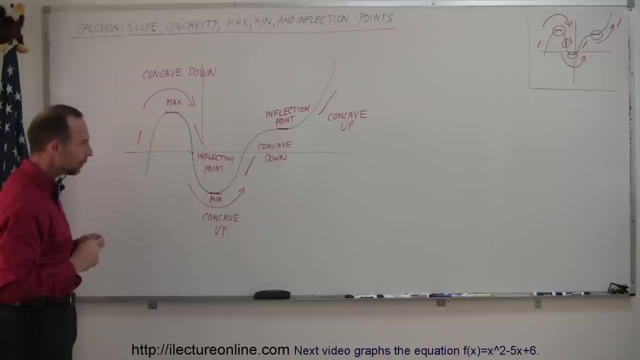 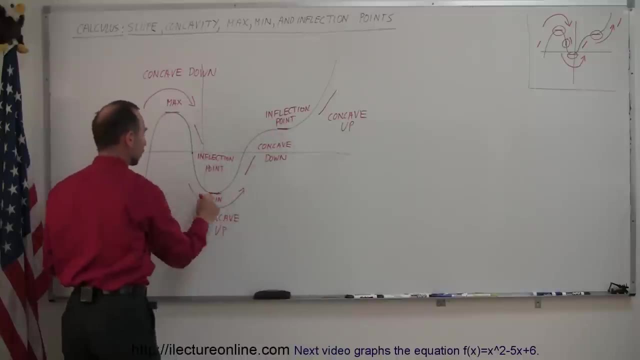 on the on the curve where the slope is zero, which means that when you find a place on the curve where the slope is zero, you're not sure if you found an inflection point or a max or a min. so you'll have to do some additional tests to figure that out. 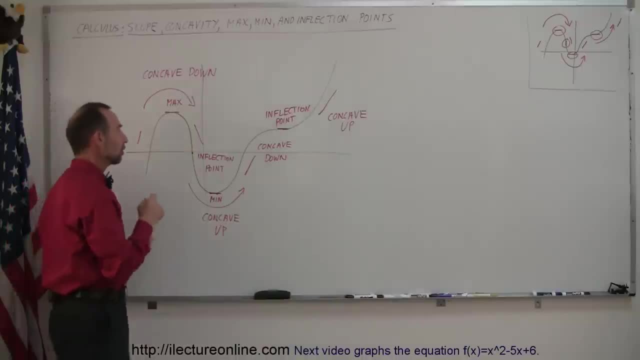 if you find an inflection point. you're not sure if you find this type of inflection point or this type of inflection point. so again, you need to do further tests to figure out which inflection point you're dealing with. so this at least gives you a pretty good feel of what we're trying to do when 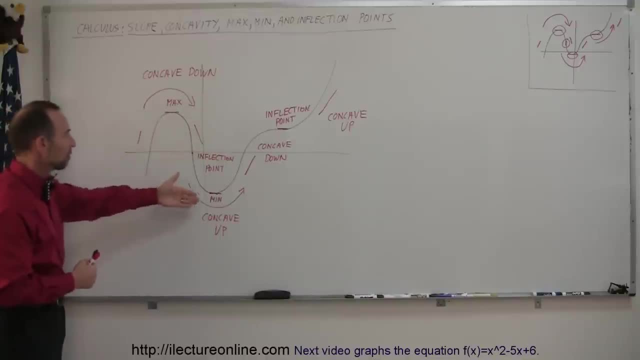 we try to evaluate a curve when we're looking for maximum points, minimum points, inflection points. this is what what i would call a horizontal inflection point. this is a non-horizontal. i would call aன Batman in this particular case. here we take a slope. we, southwestern, called a